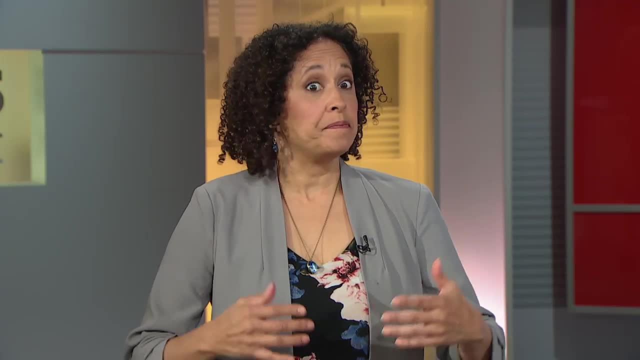 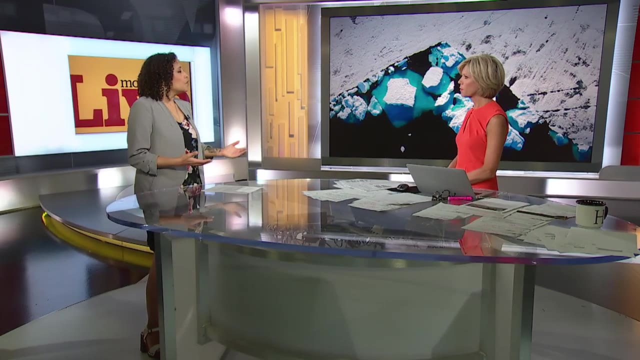 So that includes agriculture, forestry. We see forest fires continually, And look at what happened last week in the Arctic as well, So we need to actually do better at the way we're managing that, Because without it, we could face food scarcity. 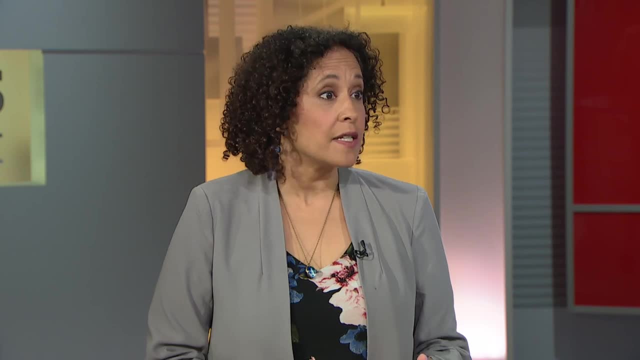 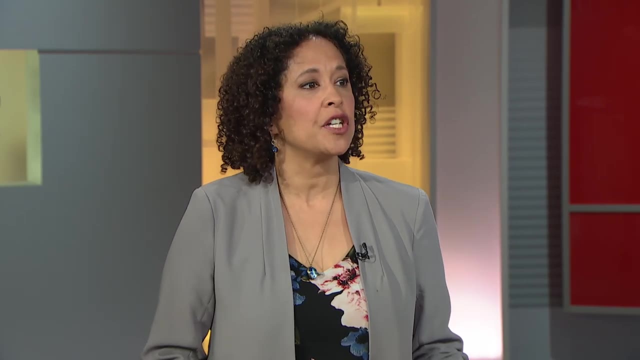 And that will end up with higher food prices, decreased nutritional value, And this is all something that we really need to take seriously. We can't combat climate change solely on reducing fossil fuel emissions. So here's what Valérie Masson-Delmotte had to say. 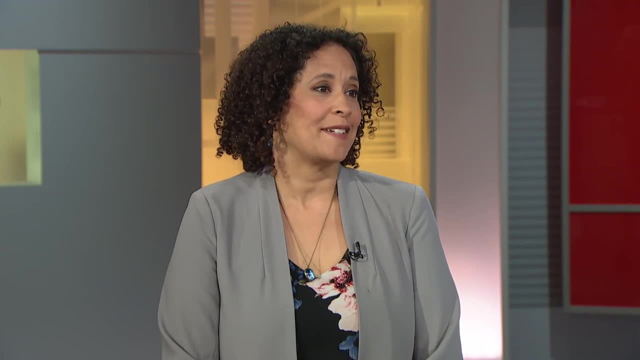 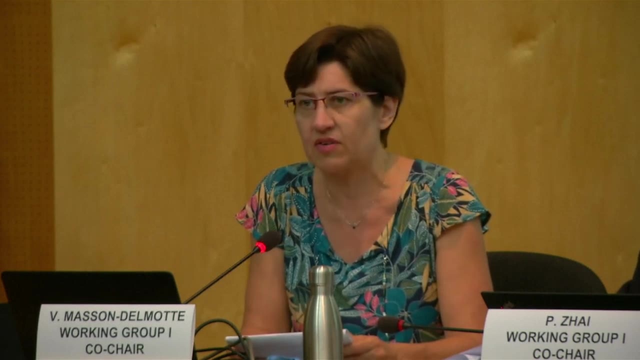 She's the IPCC co-chair and this is what she had to say about it. The way we produce food and what we eat contributes to the loss of natural ecosystems and declining biodiversity. When land is degraded, it reduces the soil's ability to take up carbon, and this exacerbates climate change. 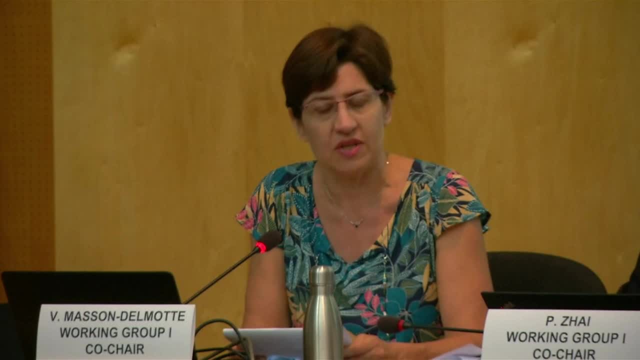 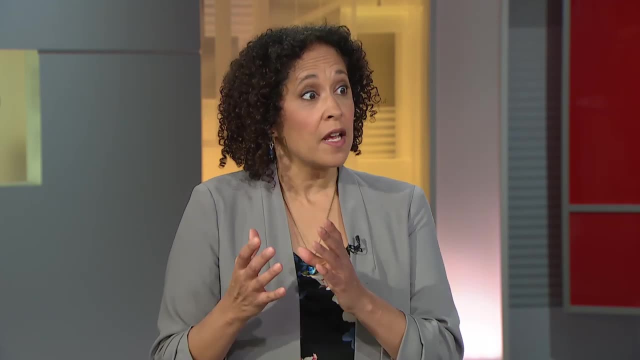 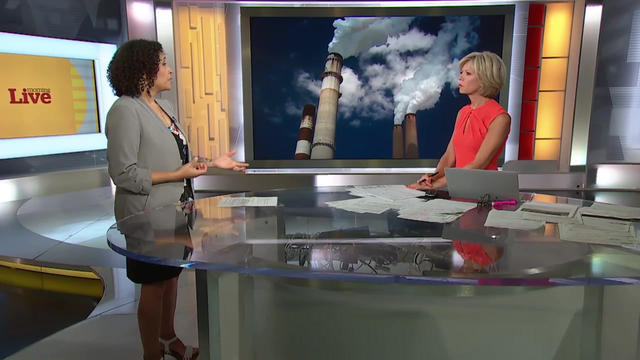 In turn, climate change ends Exacerbates land degradation in many different ways. So the thing that was really important, as was mentioned, is that our land acts both as a carbon sink and also a CO2 emitter, So this is what's really important for us to maintain: to maintain that balance. 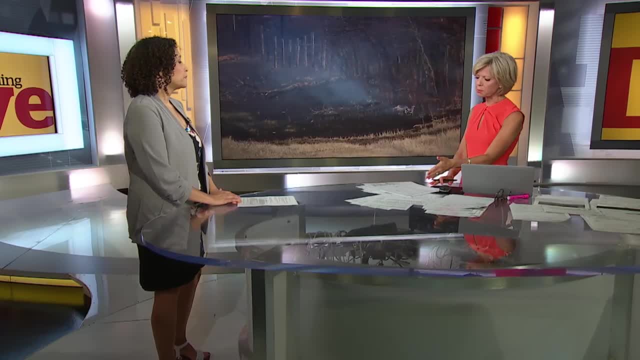 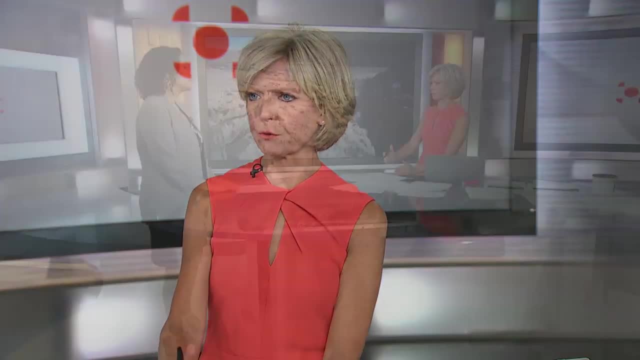 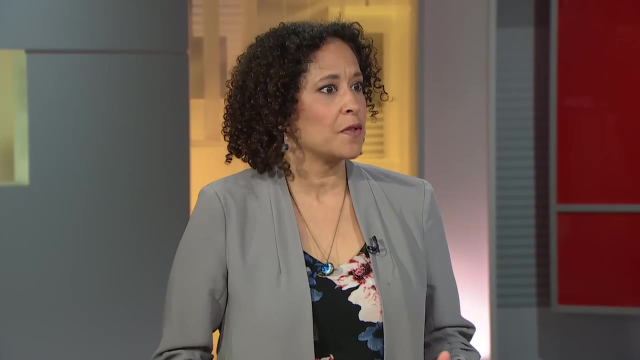 Okay to figure out how better to manage land use- Pretty stark depiction of how badly humanity is doing that. Also, they're looking to the future- Recommendations for change, And what again stands out for you in the recommendations You know, for me, even as just somebody who's guilty of this as well, is food waste. 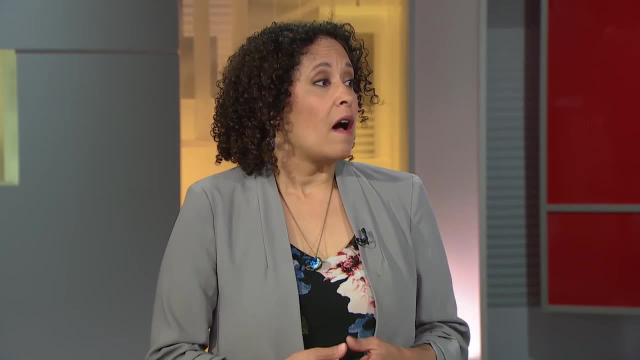 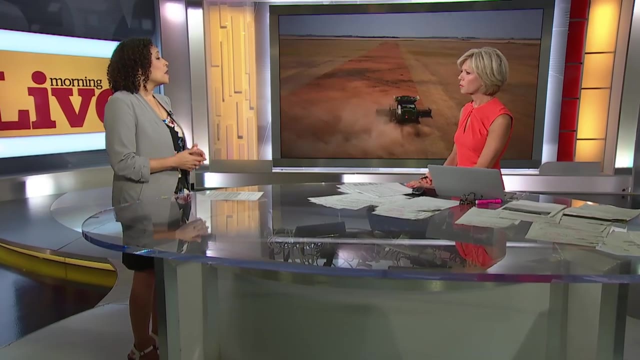 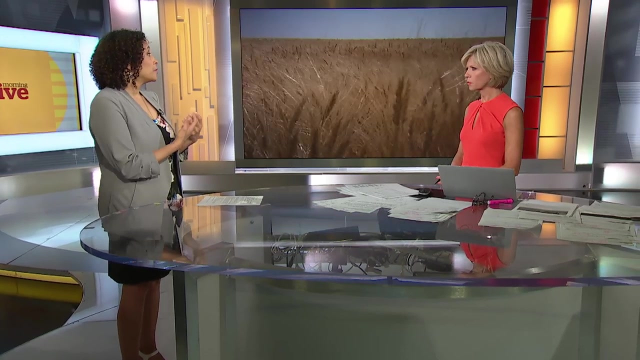 That is something that's really big As well. they're recommending shifting- we've heard this before- to a more plant-based diet, But they're not saying to get rid of meat. They're suggesting perhaps going to animal-sourced products that are sustainable and that produce less greenhouse gas emissions. 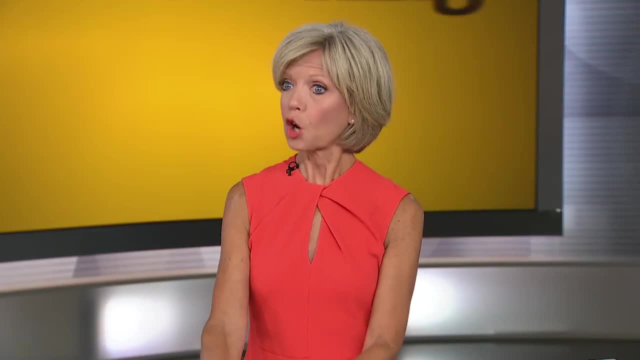 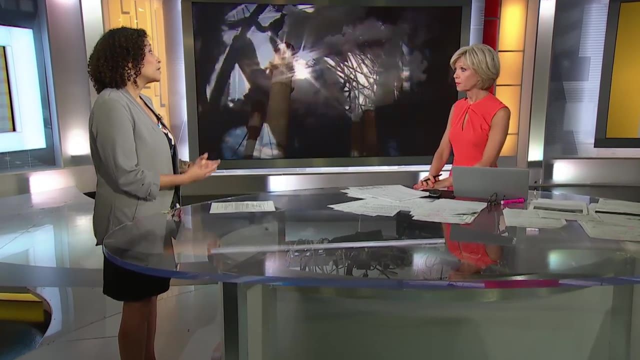 Okay, So some pretty- I mean that's common sense- day-to-day changes that humanity can make but must make, I guess Exactly. And also they're calling on governments to support the changes because, yes, they could be. the upfront cost could be costly right now. 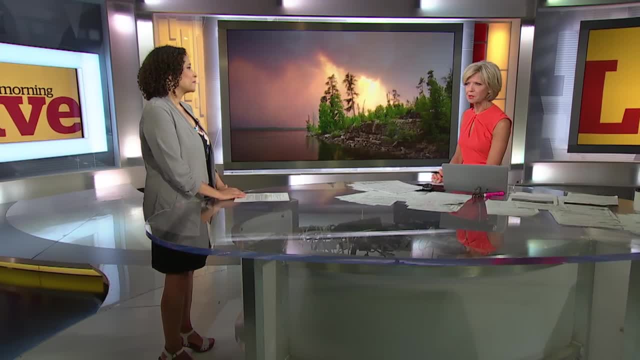 Okay, Nicole. thank you very much. An important new report out just this morning. Nicole Mortellaro here in studio with me.